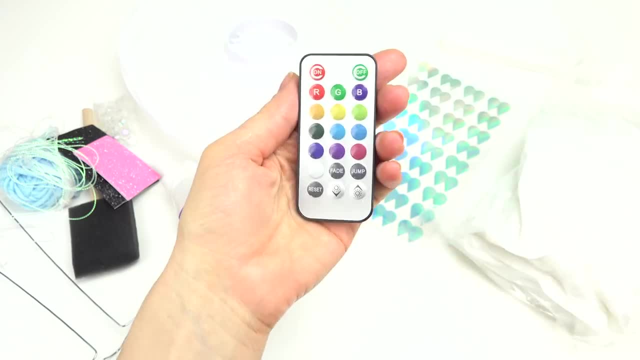 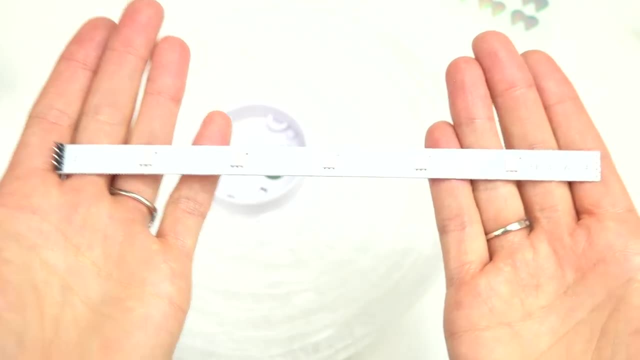 And guess what? This lamp actually works and it has a bunch of colors You can pick from. Let's make our cloud lamp. Put some batteries in here. first, This comes with an LED strip. This is what makes the lamp light up in different colors. 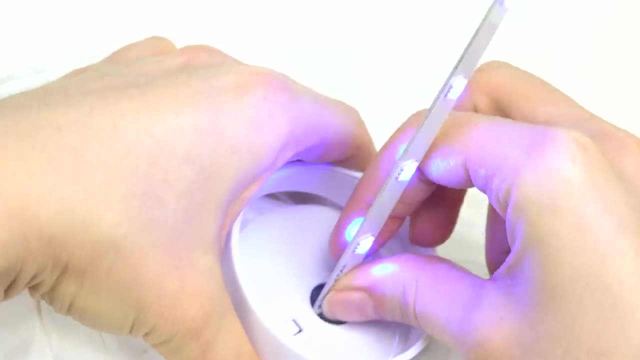 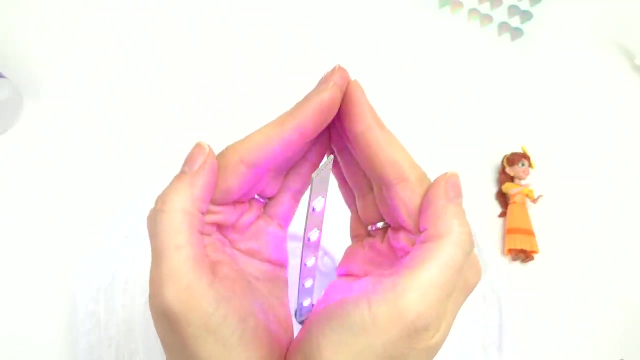 All right, put these pieces right inside of there. All right, this can be a little bit tricky, but ask somebody for help if you need it. Oh my goodness, that is so cool. Do you guys see the different colors? All right, let's raise this up. 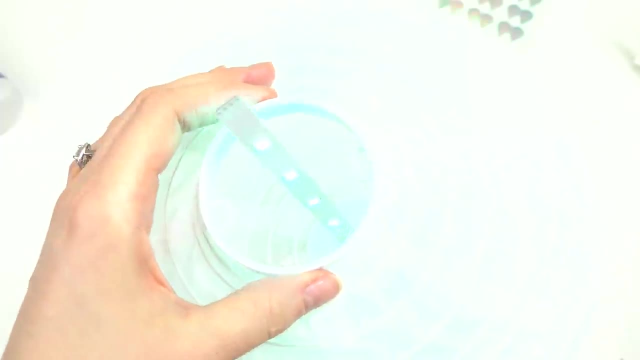 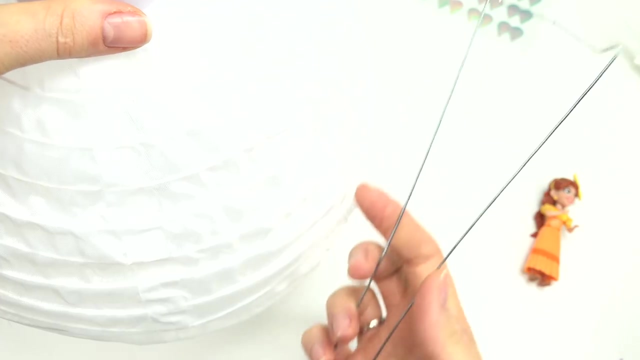 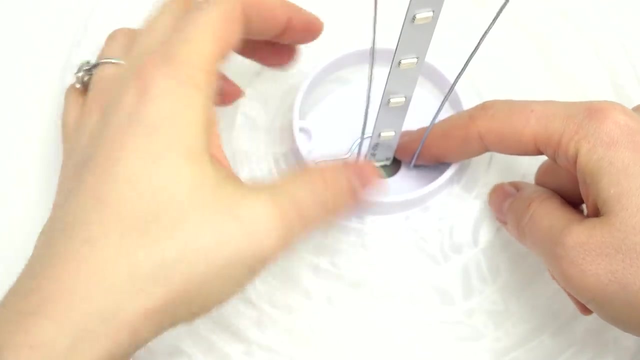 This is going to be whatever color you want it: Green, pink, turquoise, blue. Let's go ahead and shut that off for now. Now stretch your lantern all the way up and we're going to insert this metal piece for support. Okay, first I'm just going to bring it down, because the base has to go right here. 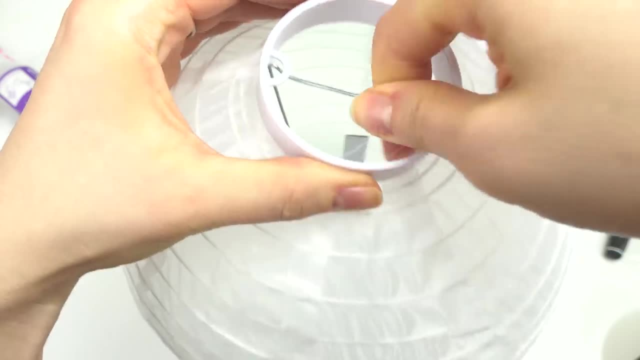 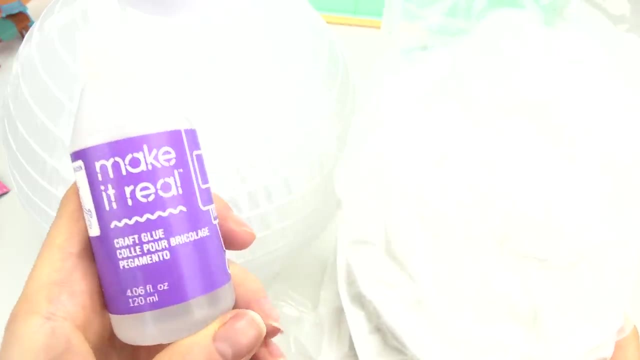 Okay, now we're going to bring it up and attach it to these holes. Now we have a lantern that we can decorate: Cloudy skies, cloudy skies. Oh, we're going to put this fluff all over it. Grab your glue and our fluff. 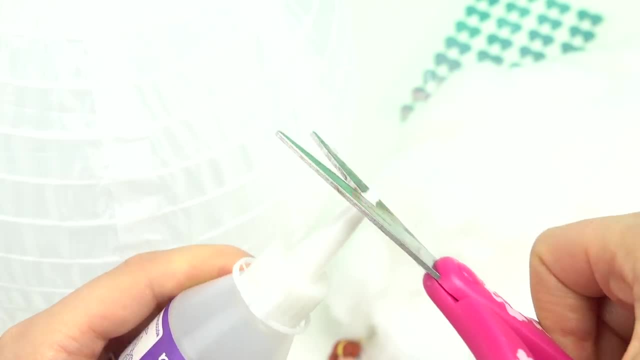 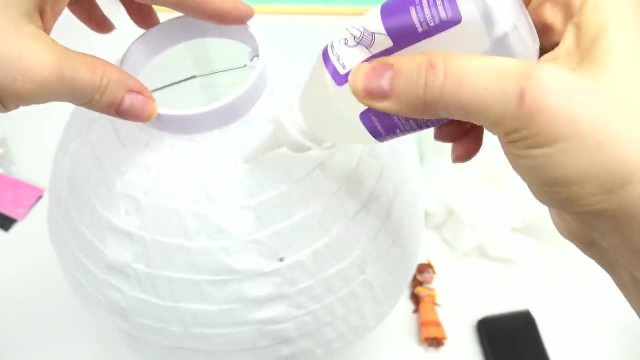 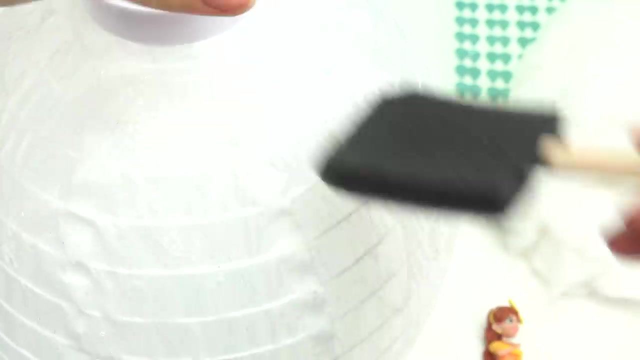 Let's go ahead and dump all of that. Oh, this is going to be so much fun. We're going to grab our brush. We're going to go ahead and put glue all over it. So start with the top half, Grab your brush and just kind of smear the glue all over. 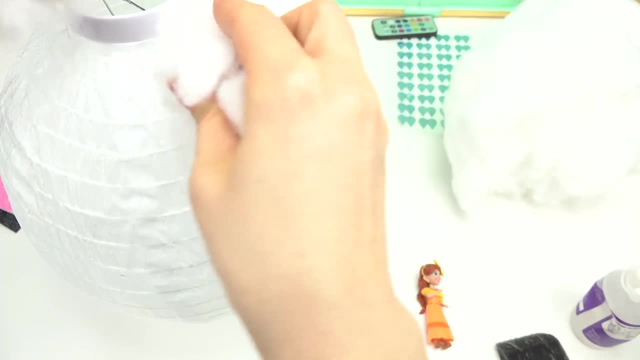 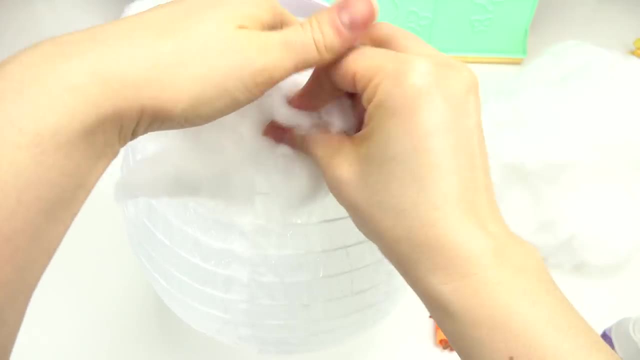 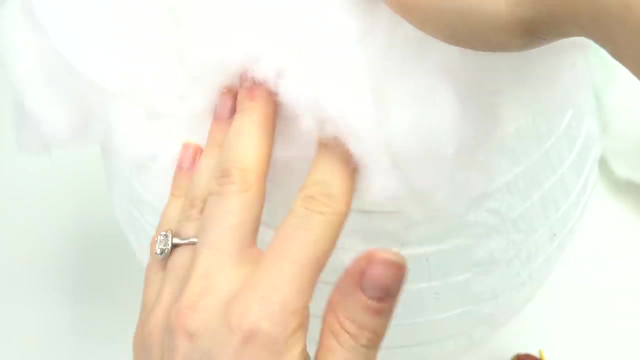 Now what you're going to do is you're going to grab just pieces of fluff and put it on the glue, And we're going to do this all the way around And make sure it's stuck on the glue, Okay- And then we're going to press it down right here. 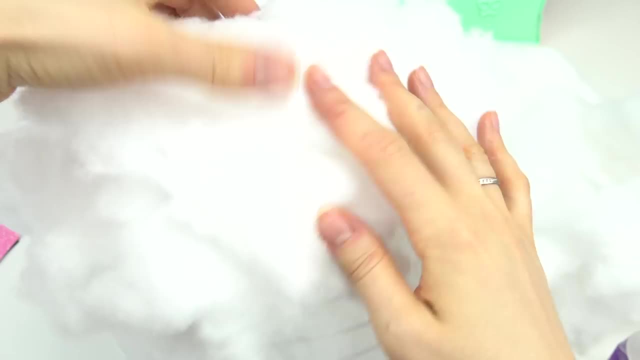 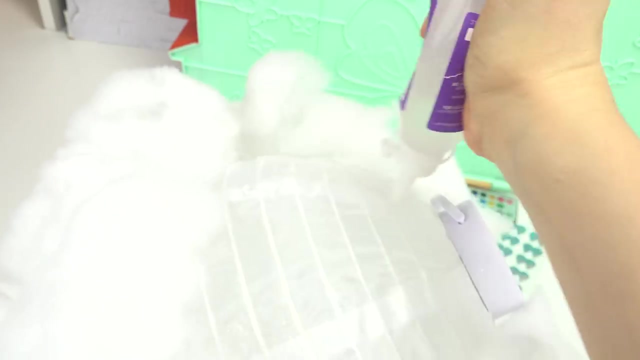 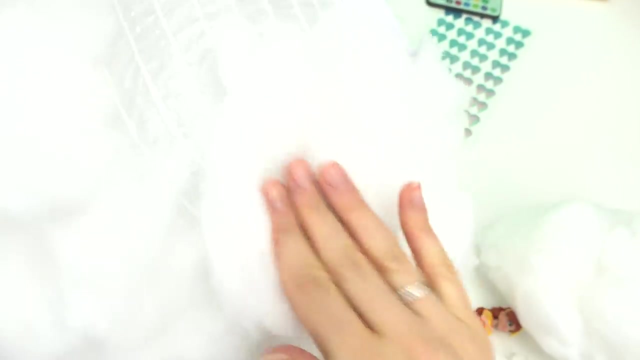 It's going to look fabulous. All right, What do you guys think? so far, We're going to keep on going. We've got one small spot left. Smear that glue again. I'm going to put these last pieces on here. 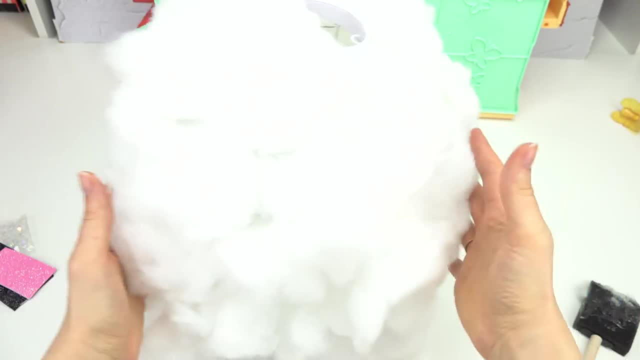 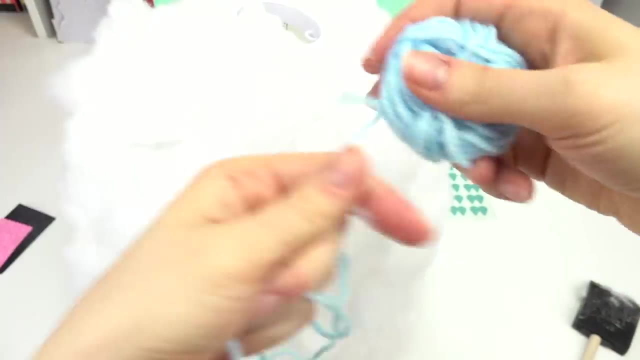 So this is what it looks like so far. It literally looks like a cloud. Now we're going to take some yarn and we're going to wrap the whole entire cloud Land Turn in this. I'm just going to go ahead and just wrap it around the whole entire thing. 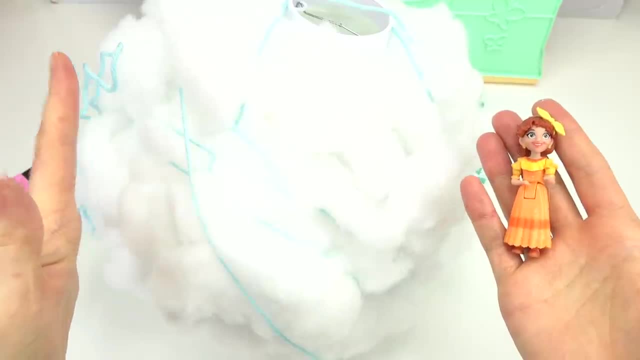 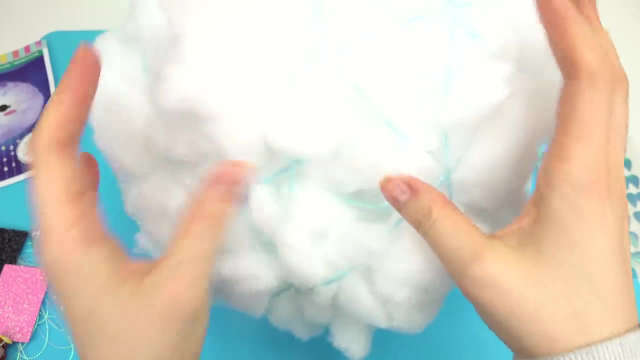 Just go in different directions. Now I'm going to let this dry for three to four hours, and I can't wait for the rain. All right, It's been two hours and the glue has hardened, So what I'm going to do is I'm going to remove all of this yarn that I have wrapped around. 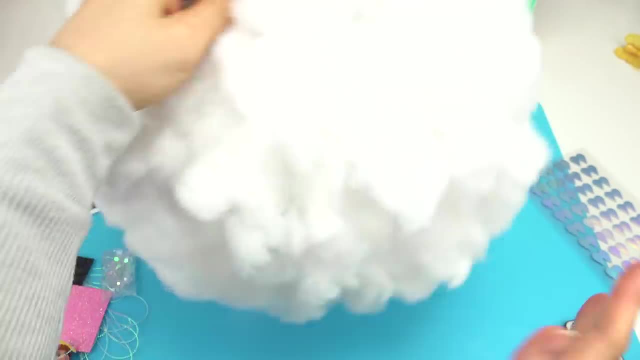 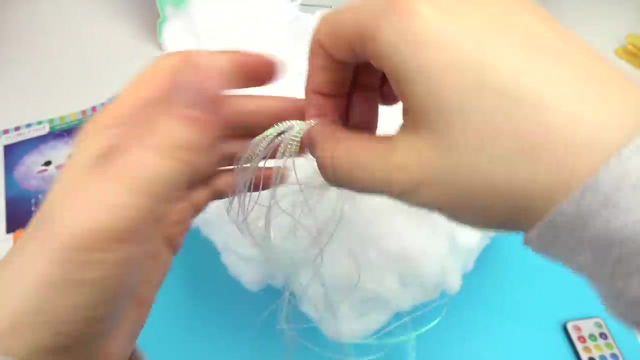 This is what our lamp looks like so far. It's so fluffy and it looks awesome. Next step: We're going to Take this cord and we're going to start cutting this. This is used for the raindrops that are going to come down from the cloud. 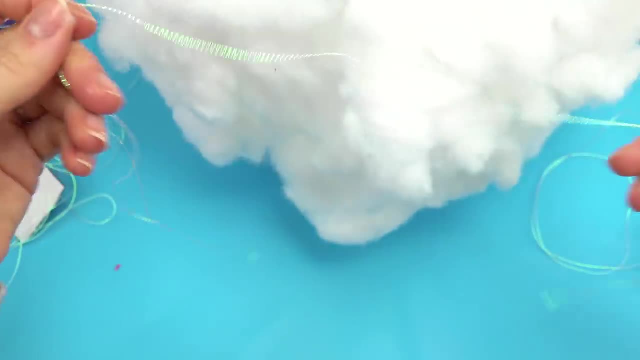 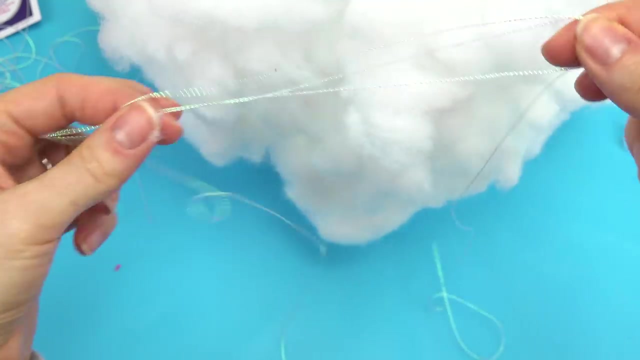 So I'm going to cut about 23 inches. This is going to be used to hang up our lantern. The next cord is going to be used to wrap this around so that the raindrops can fall down. Next, I'm going to cut nine cords. 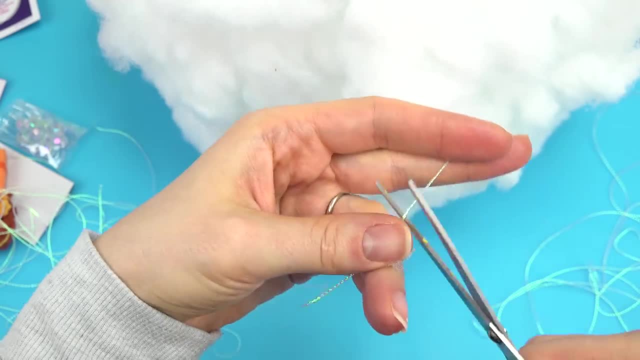 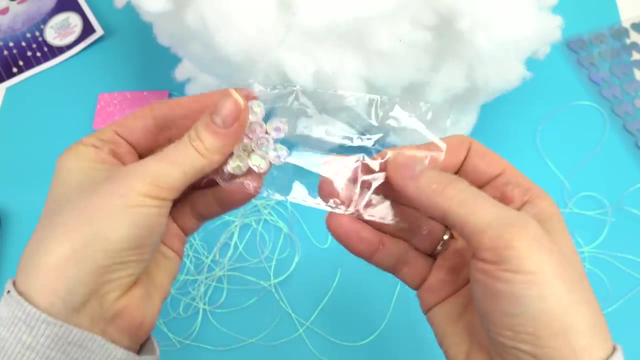 They're about 25 inches each, and this is where the raindrops are going to hang off of. I see the clouds coming in. Now that we have All the cords cut up, we're going to put these colorful beads on each of the nine strands. 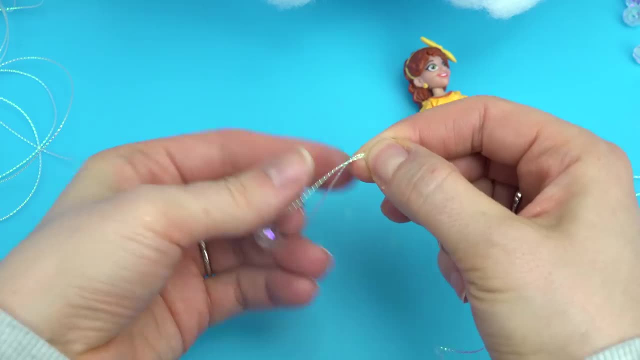 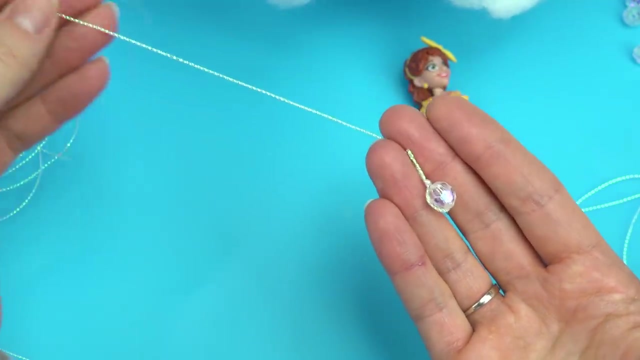 Go ahead and pull that through, And now I'm going to make a double knot. All right, There it is. This is going to help weigh down all of the raindrops that we're going to put on the strand. All right, Last one. 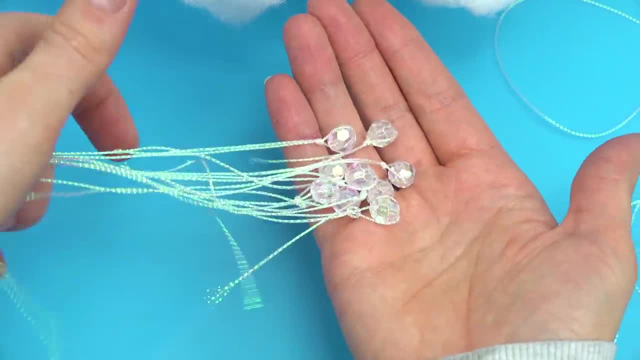 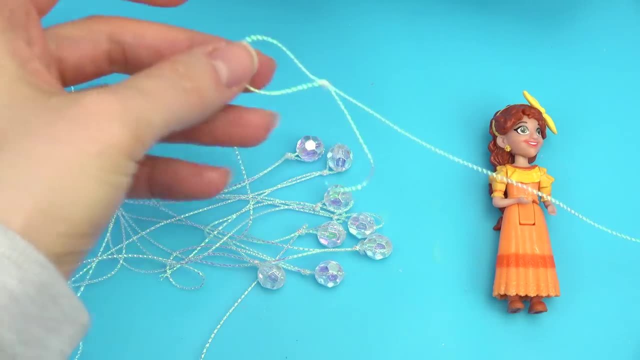 Now we have these beautiful shiny beads. They look like raindrops. Did somebody say rain? Did somebody say rain? For each of these nine beads, I also made A double knot on the other side of it and that's going to be used because we're going. 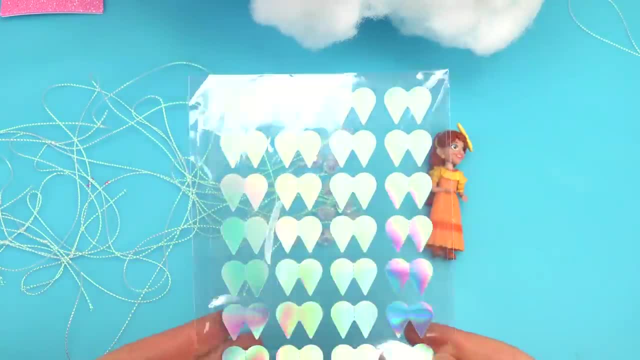 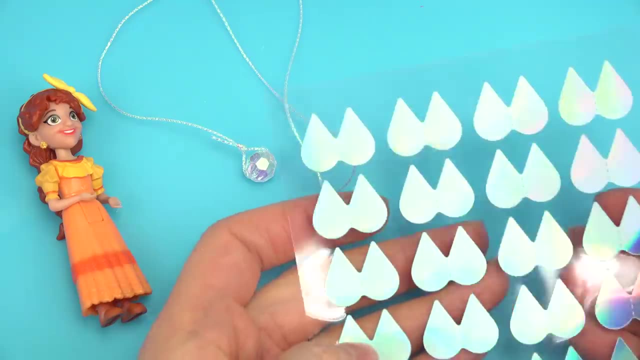 to put it around the cloud. It's raining up. next, We're going to put these raindrop stickers on each of the cords, So let's take one of them. This is what they look like: They're raindrop stickers And like when I move it, it changes colors in the light. 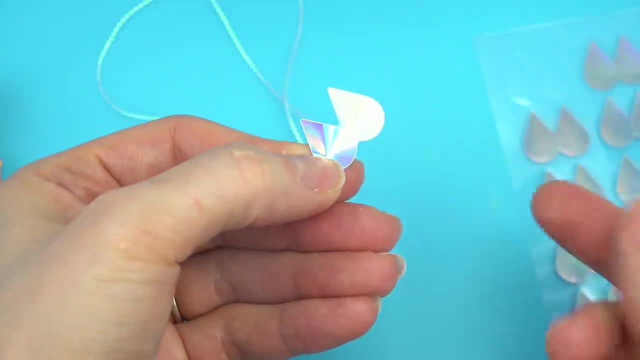 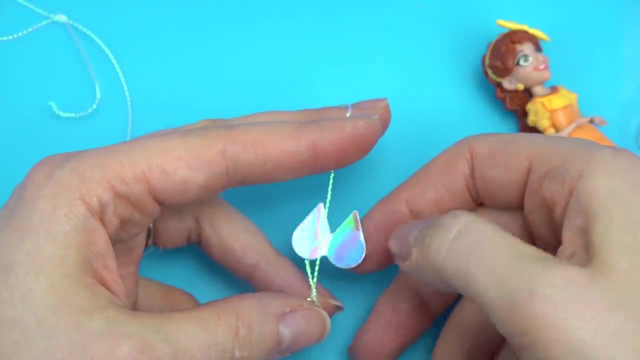 Let's go ahead and peel one back, And each of them has a double line so you can fold it over. So what we're going to do with the sticker is you're not going to put it where the bend is. Put it in the middle of the raindrop and fold over your raindrop sticker. 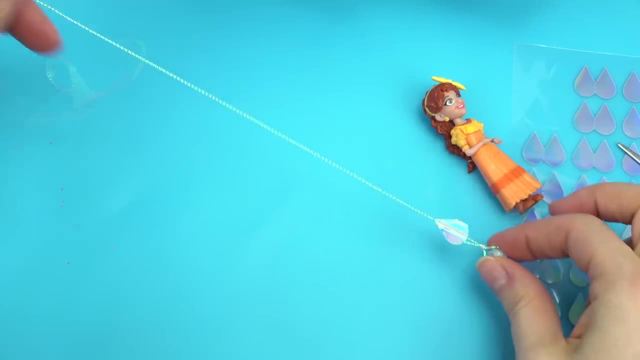 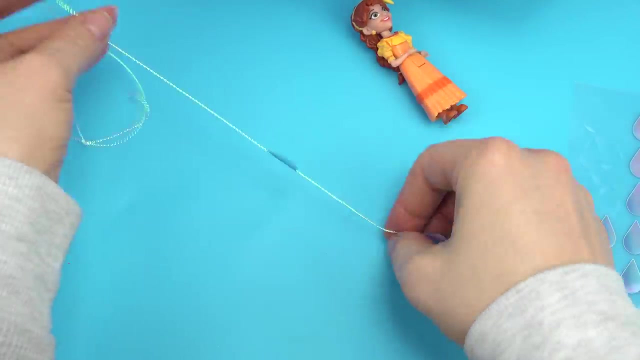 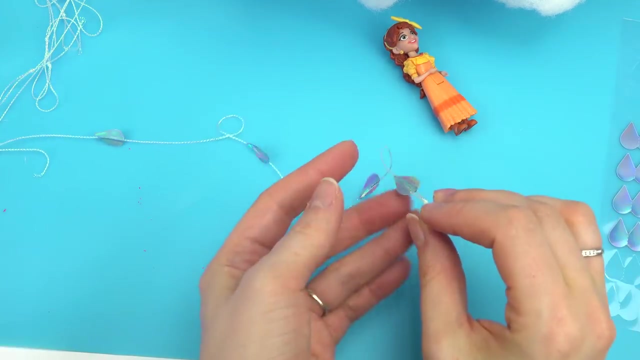 So now it looks like the rain is falling down, We're going to add four of these sticker drops to each cord and make sure you space them out a little bit. This is what the strand is supposed to look like, So the bead weighs down each of these raindrops. 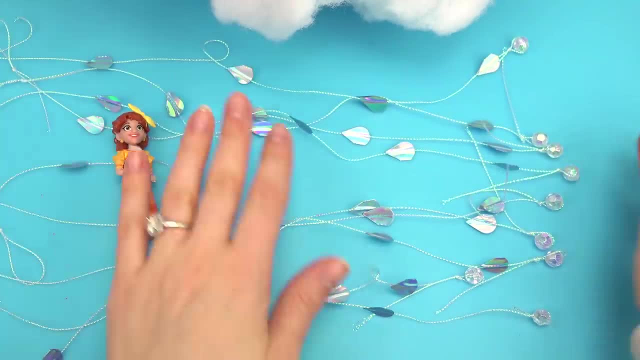 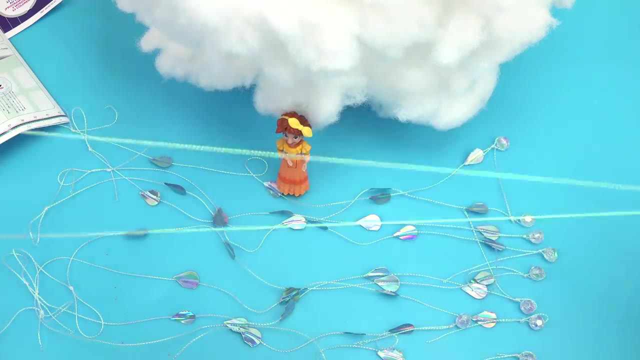 All right, Here's the last one. Now we have nine strands. Raindrops keep falling on my head Up. next, we're going to take our longest cord that we cut and we're going to thread each of these nine strands in it. 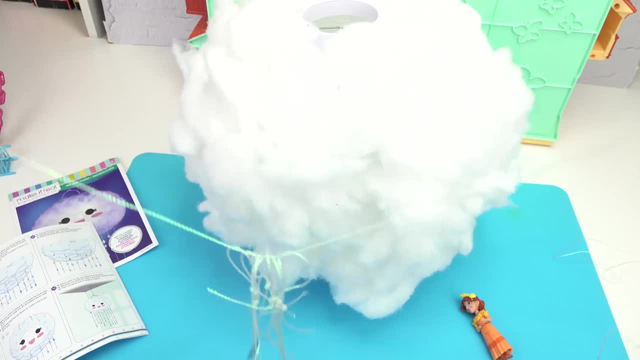 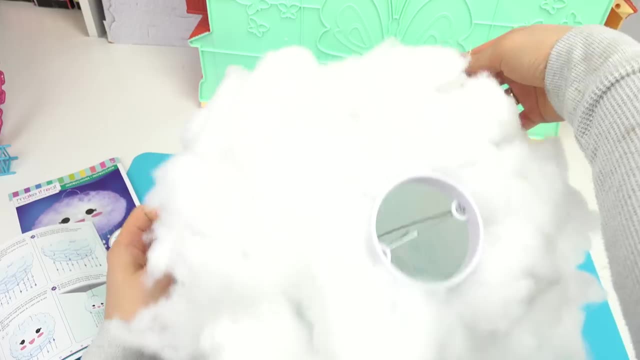 So this is what it looks like so far. They're kind of all clumped together, But once we wrap it around the lantern then we can kind of adjust them. So let's go ahead and do that. You're supposed to wrap it around the middle. 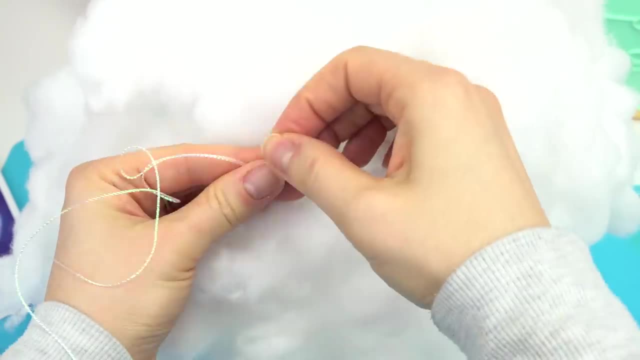 Now make sure it's really tight around it so that the raindrops won't fall, And then we're going to take our longest cord that we cut and we're going to thread each of these nine strands in it, And then we're going to tie it around our cloud. 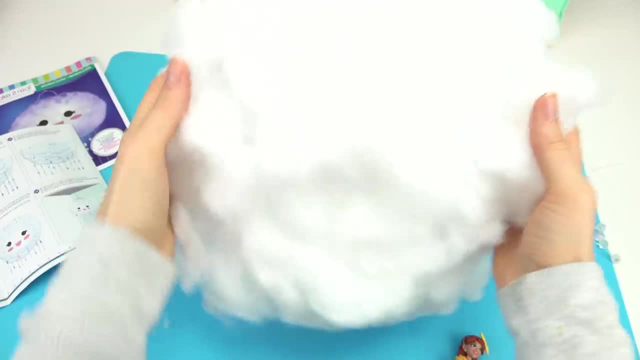 And then we're going to tie it around our cloud. This is going to be a little bit more painful And make a double knot. Cut any loose ends, And you could always fluff it up a little bit to hide the string. All right, where are the raindrops? 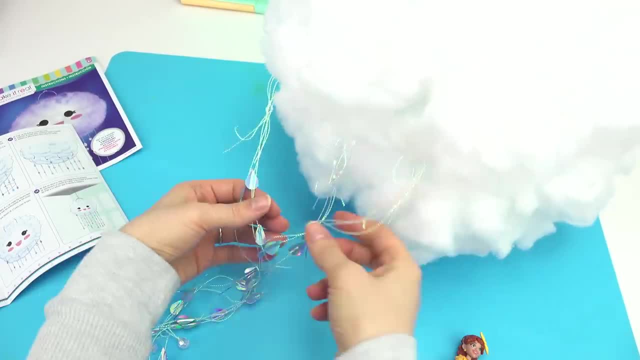 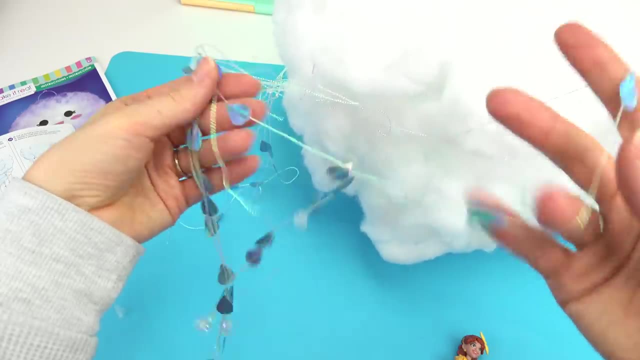 So here they are. I'm going to go ahead and just adjust them around our cloud. They might be stuck together. So just be really careful. All right, Here we go. One's going to go over here. You could either put all of them kind of in the front of your cloud or just throughout. 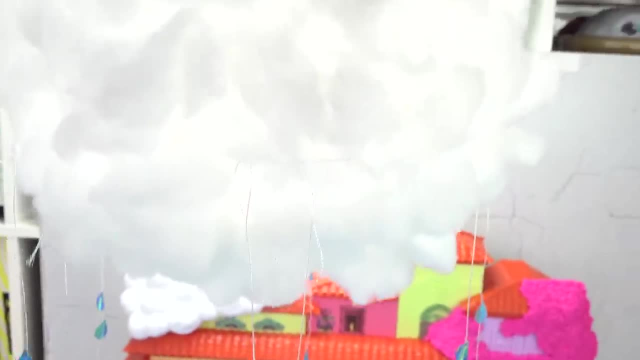 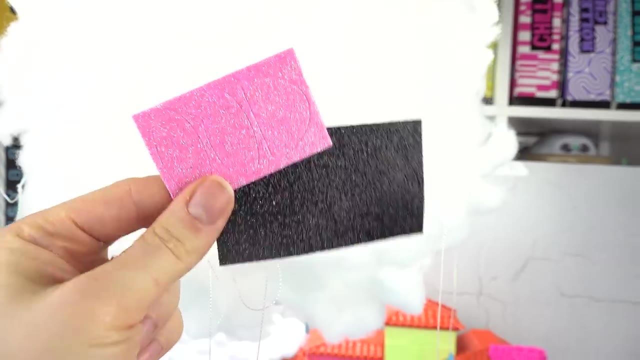 the whole thing All right. Kaboodle fans what it looks like so far. we've got this huge fluffy lamp raindrops coming down on our madrigal house. now we need to decorate it. i'm gonna put some eyes on it. there's one. how kawaii are these? 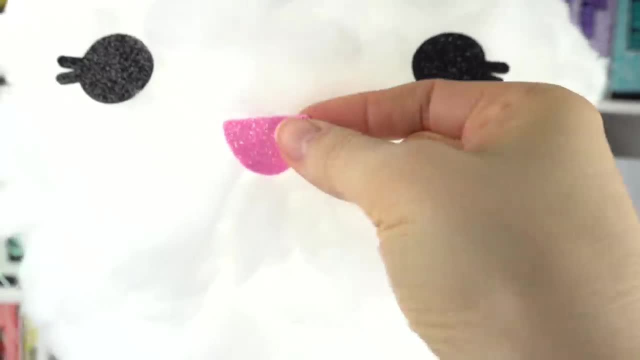 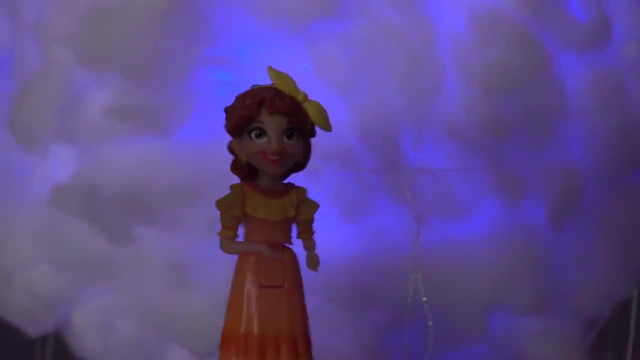 and you just literally stick them on the fluff. i have this cute pink mouth. there we go, and, of course, some cute cheeks. fun. i can change the color of the cloud based on my mood. that's right, caboodle fans. i've got this remote and then we could switch the cloud to whatever color we want.